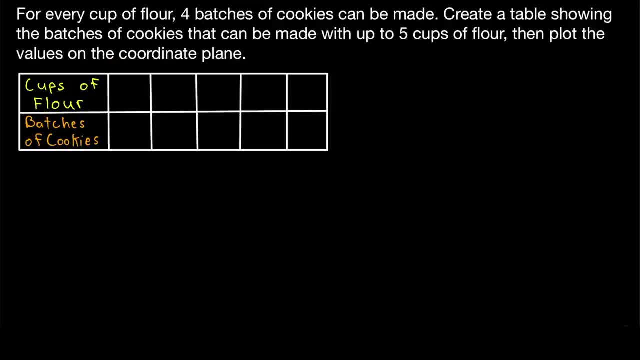 coordinate plane. Remember that a ratio is just a way of relating two quantities. In this problem, we're given a ratio that with one cup of flour we can make four batches of cookies, And I'm going to show you how to do that. So let's get right into it. 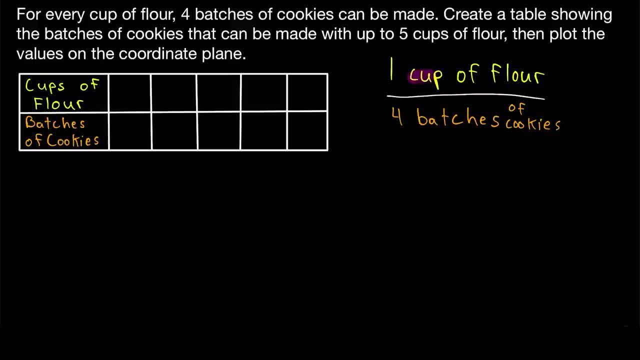 Oftentimes, if we already know the quantities being related- in this case cups of flour and batches of cookies- we don't have to write the units every time, So we might write this ratio in a more compact form as just one over four To create a ratio table. we create one row. 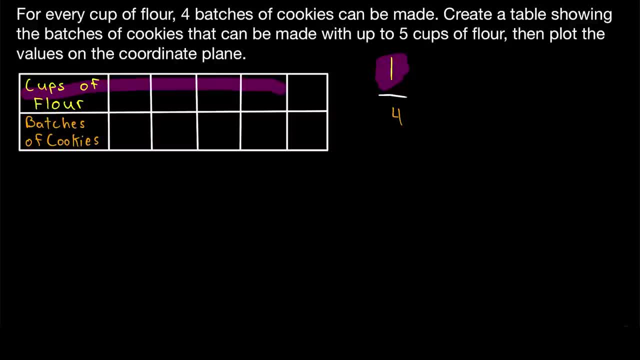 for the top quantity in our ratio, in this case cups of flour, and then another row for the bottom quantity, which is batches of cookies. in this case, We title the rows in the first column so that we know what types of quantities we're relating. 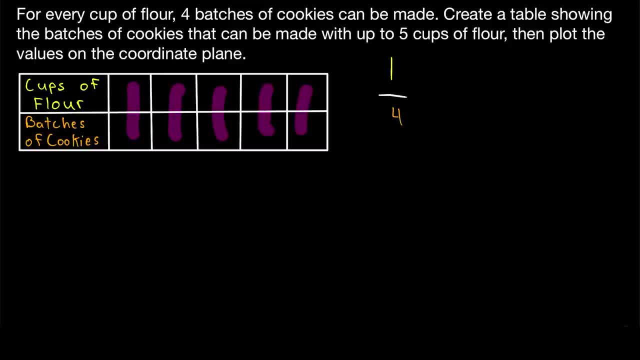 and then in the other columns we can express equivalent ratios between the quantities. So for example, in the first column we would put our given ratio that with one cup of flour we can make four batches of cookies. Then you may recall, I went over this in my first lesson. 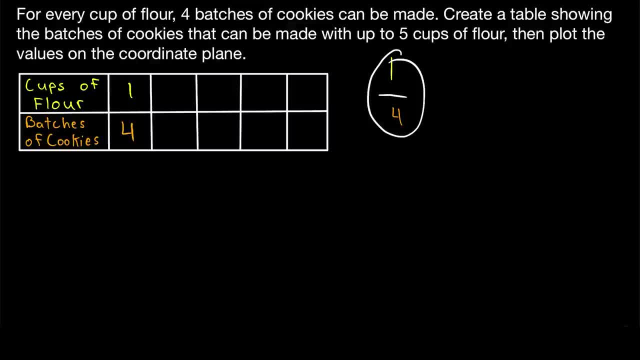 on ratios. We can scale ratios up or down. For example, if we multiply the number of cookies, multiply the top number by two and the bottom number by two, we'll get an equivalent ratio of two over eight. So if one cup of flour is enough to make four batches of cookies, 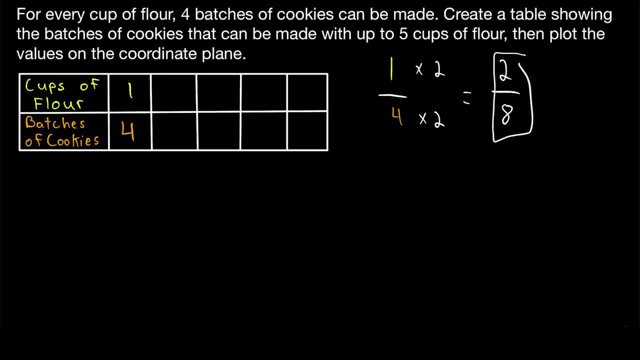 that means that two cups of flour is enough to make eight batches of cookies. By scaling ratios up and down in this way, we can fill in a ratio table to find specific ratios that we're interested in. In this case, we want our table to show the batches of cookies. the 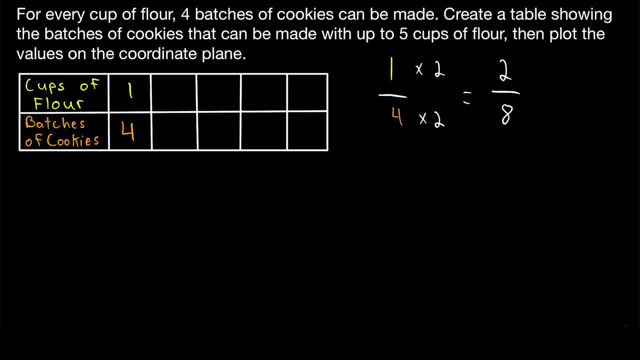 can be made with up to five cups of flour. So let's continue scaling our ratio. We just scaled our first ratio by multiplying both quantities by two, giving us this new one that we can now put in the table. For two cups of flour, we can make eight batches of cookies. As a quick reminder, 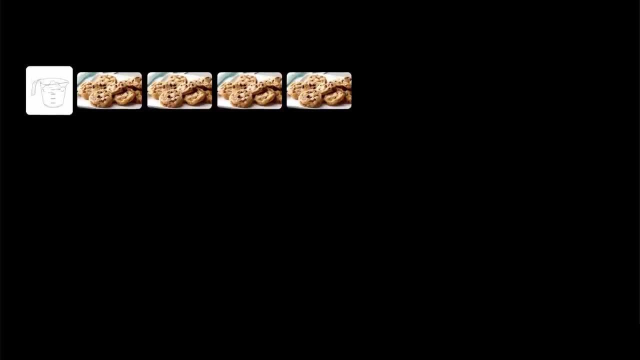 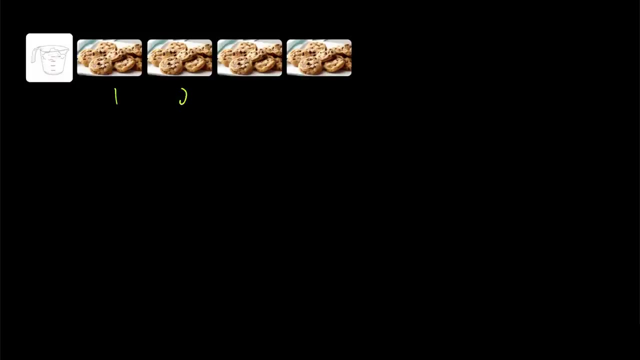 of why we can scale ratios in this way. let's just take a look at this picture. This expresses the first ratio. we saw that for one cup of flour we can make one, two, three, four batches of cookies. So that's a ratio of one to four. Remember that this is another way we might express that. 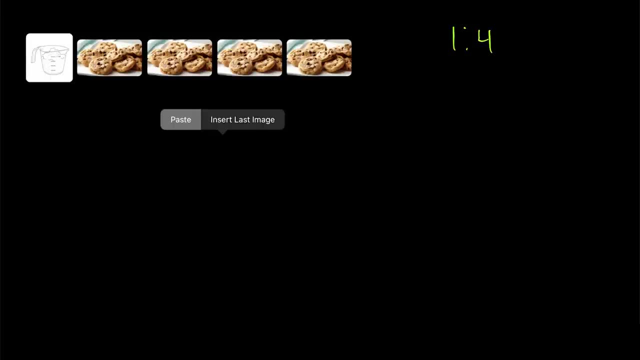 ratio. Then to scale the ratio up by a factor of two, we could just make a duplicate of this picture to get a visual of what that looks like. And now we see that ratio that we saw above. For two cups of flour, we're able to make eight batches of cookies. 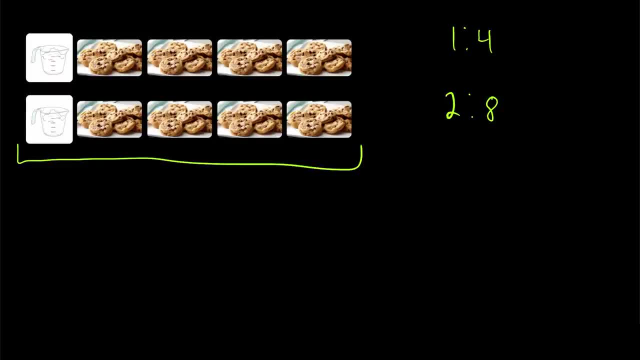 What I want to point out is that even after we scale this up, this picture still expresses the first ratio as well. It's still the case that for every one cup of flour, we get four batches of cookies. We can see that quickly by counting. We've got one cup of flour, one. 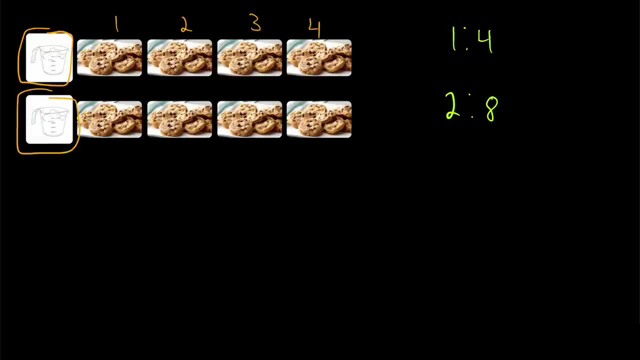 two, three, four batches of cookies, another cup of flour, one, two, three, four more batches of cookies. So even after scaling the ratio up, it's still the case that for every one cup of flour we get four batches of cookies. just wanted to provide a visual to help justify. 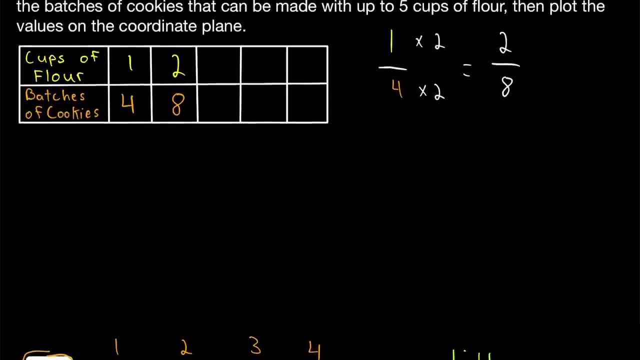 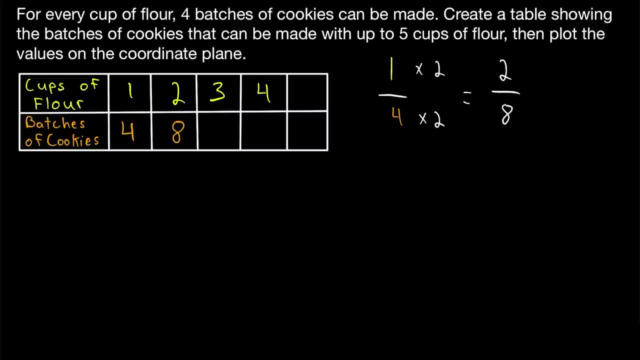 why this makes sense. Now let's head back to our ratio table and quickly finish this up. All we have left to do is figure out how many batches of cookies we can make with three, four and five cups of flour. One way we could figure out how many batches of cookies we can make with three cups of: 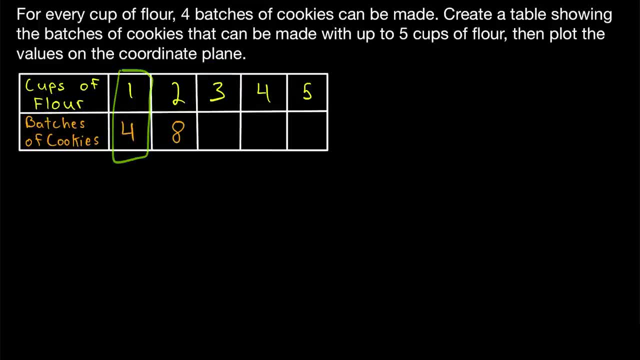 flour is to just scale up our original ratio. We know the ratio is one to four. Then if we scale this ratio up by a factor of three, so we multiply both quantities by three, we'll see that for three cups of flour we're able to make 12 batches of cookies. 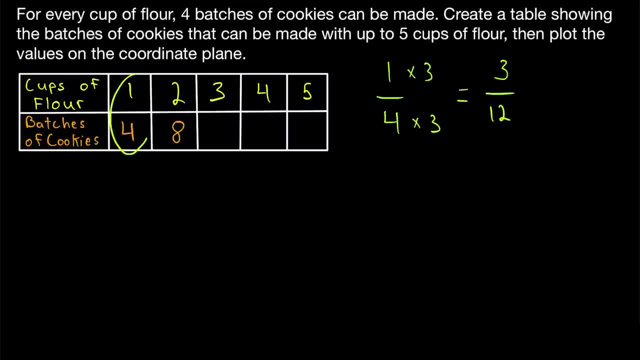 That's four times three. However, instead of using multiplication to get from this ratio to this ratio, we could also just use addition to get from this ratio to this ratio, because going from two cups of flour To Three cups of flour is an increase by one cup of flour, and we know from our original. 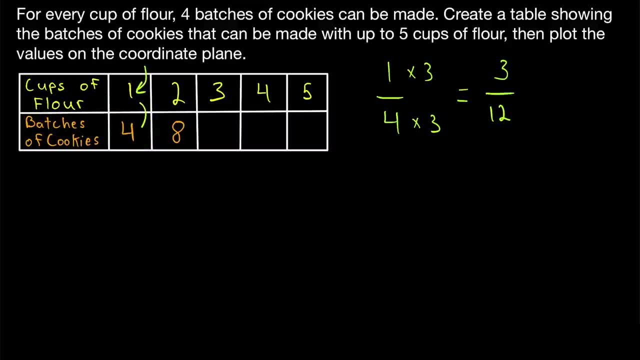 ratio that for every one cup of flour we add, we can add four batches of cookies. So if we go up by one cup of flour, we would need to go up by four batches of cookies and we would arrive at the same answer. we just did that three cups of flour will be enough. 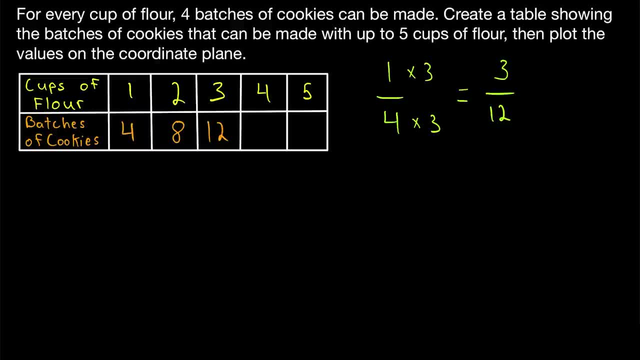 for eight plus four or twelve batches of cookies, and we could do the same thing to get From here to here. if we go up by one cup of flour from three to four, then to keep the ratios equivalent we need to go up by four batches of cookies. so twelve plus four, that's. 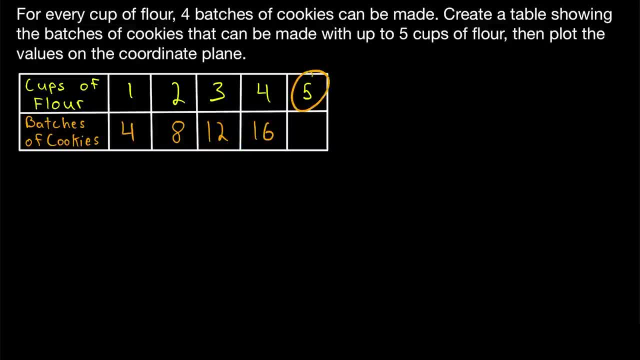 going to give us sixteen. and then finally, how about five cups of flour? how many batches of cookies can we make if we've got five cups of flour again? we could figure that out any of the ways we've already discussed. we could scale up the ratio of one to four or since. 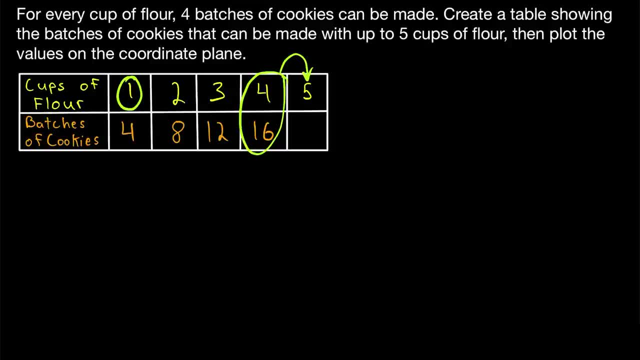 we had to add one cup of flour to get from four to five. we could add four batches of cookies to get from sixteen to twenty. but we don't always have to add this original ratio. as long as we add equivalent ratios together, we'll just get another equivalent. 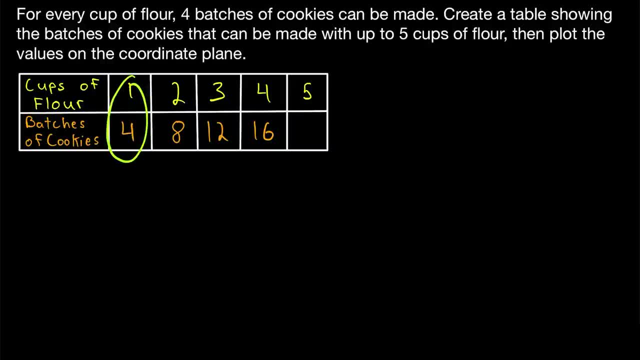 ratio. what do I mean by that? well, instead of adding one cup of flour and four batches of cookies to four cups of flour and sixteen batches of cookies, two plus three is five, and that's the last column. We've got to fill out five cups of flour. we know that with two cups of flour we can make. 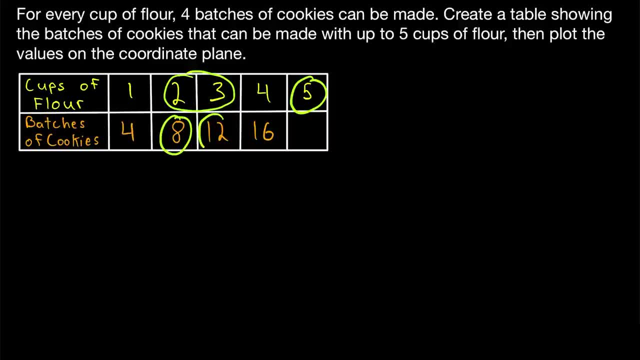 eight batches of cookies and with three cups of flour we can make twelve batches of cookies. so with two plus three or five cups of flour we can make eight plus twelve or twenty batches of cookies. so I hope that just shows you some of the different ways we can arrive at equivalent. 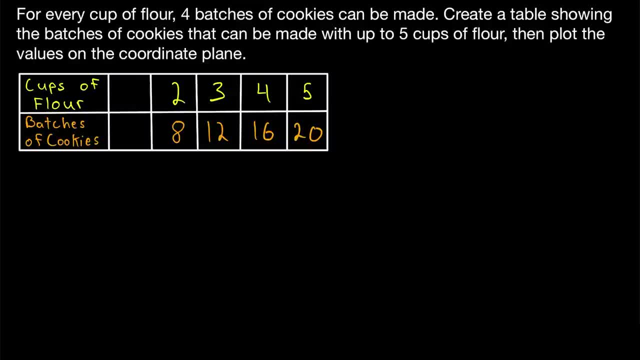 ratios that might be useful if we weren't given the original ratio and perhaps all we were given. So let's go ahead and look at these three ratios and then we want to find how many batches of cookies we can make with five cups of flour. to figure that out, we could scale either of 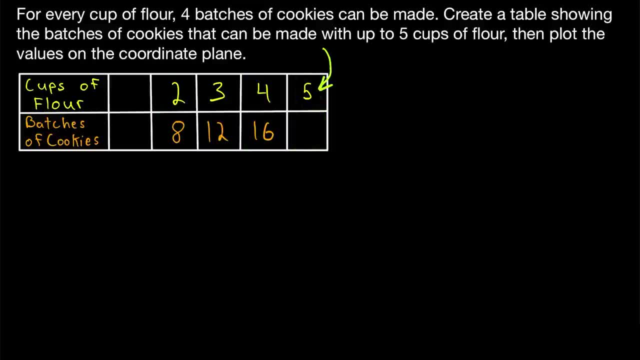 these ratios down and then scale them back up to the quantity we want. but we wouldn't be able to scale just one of these ratios up easily because none of these numbers multiply evenly into five. we could use decimals, but as long as we're trying to do this without 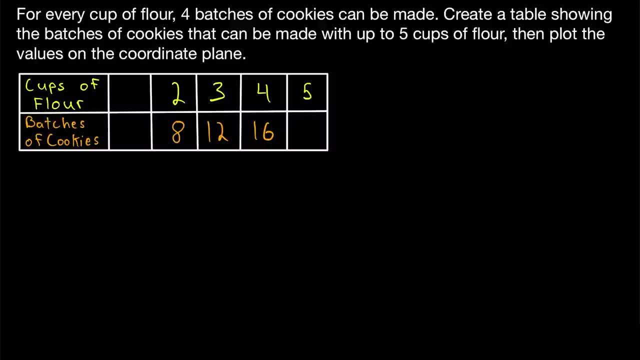 a calculator. it might be best to avoid that if possible, And so in that situation we could solve the problem by just adding these two ratios together. but enough of that. we have finished our ratio table, so let's switch over to graph paper and graph the values. 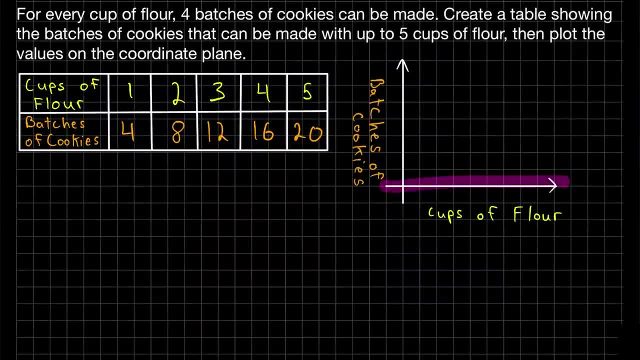 So here we've got our x- y plane. I've labeled the horizontal x axis cups of flour and the vertical y axis will represent batches of cookies. you could put either quantity on either axis, it doesn't matter, but you're probably going to be expected to put the first quantity. 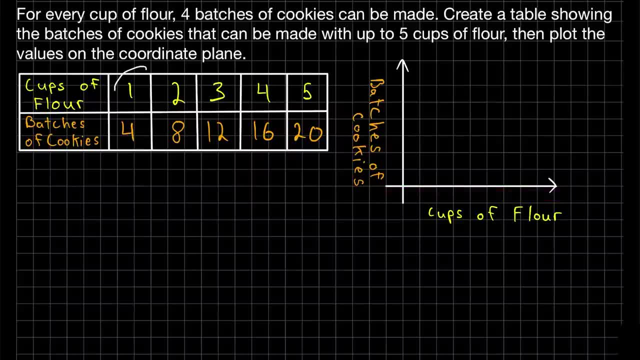 in your ratio in the x axis. since our cups of flour are just going up by one, that will work fine for our units on the x axis. so we'll start with one and then two, and then three, four and five. our batches of cookies, on the other hand, are going up by units of four. so 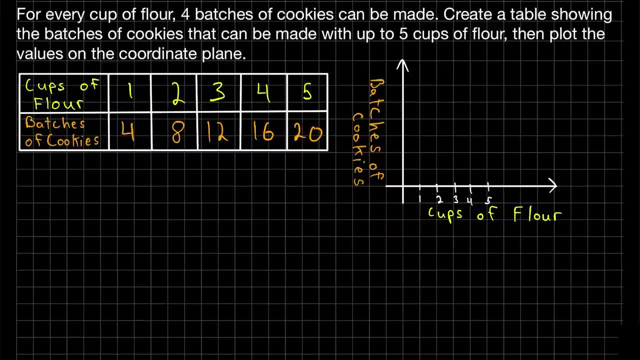 in order to make sure we have space for all of our points, let's go up by units of four on the y axis. Then, with our axes labeled, We can go ahead And plot these equivalent ratios in the plane. we know that one cup of flour will give us. 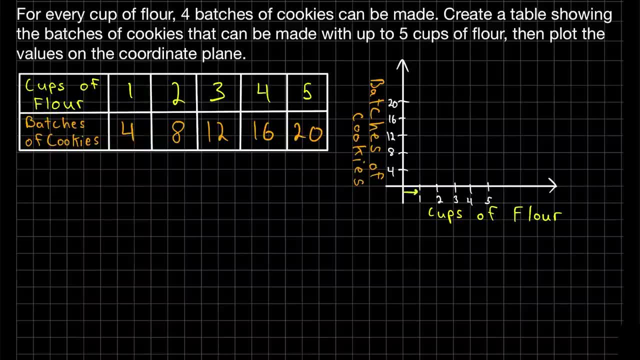 four batches of cookies. so we can plot that go over to one on the cups of flour axis and up four on the batches of cookies axis. it looks like we're going up one, but remember our units are going up by four on the y axis. so there is our first ratio: one cup of flour. 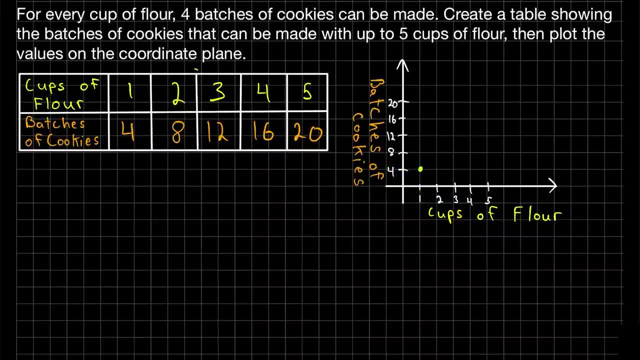 gives us four batches of cookies. and we proceed in the same way for all the other ratios. So we can plot these equivalent ratios in the plane. Two cups of flour gives us eight batches of cookies. three cups of flour will give us twelve batches. four cups gives us sixteen batches, and five cups gives us twenty batches ratio. 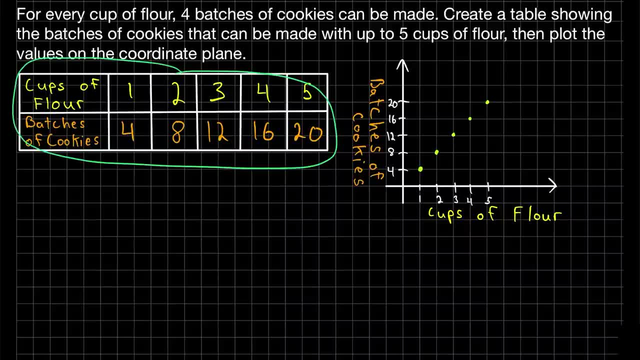 tables should consist of equivalent ratios. so when you plot your tables- values on an x- y plane, you should be able to draw a straight line through the points. of course it won't be exact because you're drawing won't be exact, but if it doesn't look like the points all. 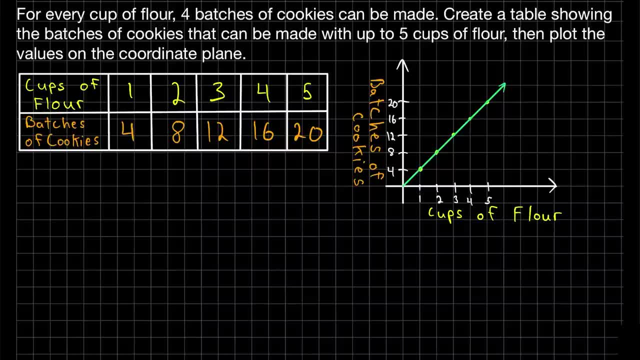 fall on a line, then you might have gone wrong and should double check your ratios. for example, if I accidentally calculated that five cups of flour could give me twenty four batches of cookies, then I would plot this point right up here and that would look like a problem. 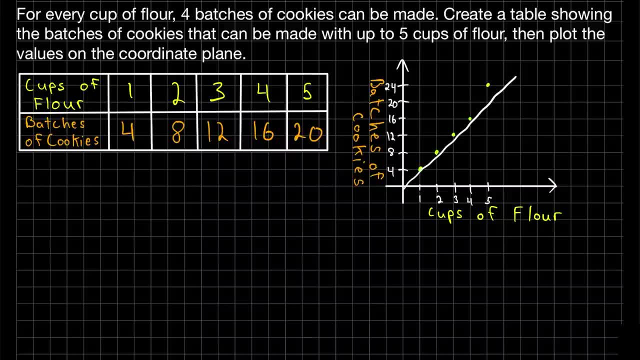 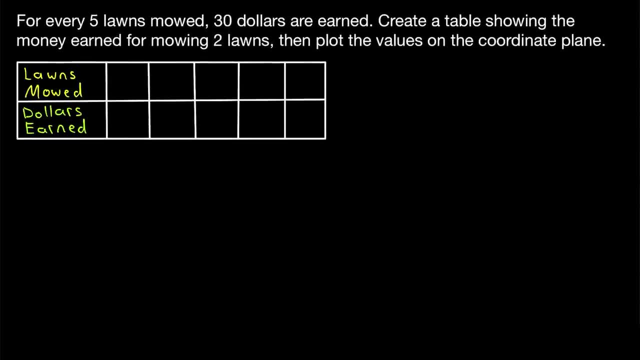 because I know I'm not going to be able to draw a straight line through all of those ratios. all right, we spent a lot of time on that one, so we're going to go a bit quicker through this second and last example problem. Really recommend giving it a try yourself before watching the rest of the video, for 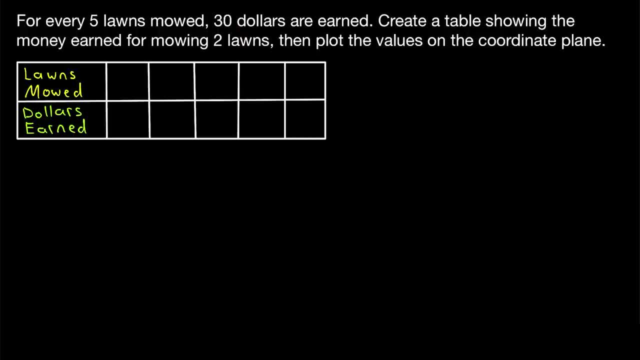 every five lawns mode thirty dollars are earned. we want to create a table showing the money earned for mowing two lawns specifically and then plot the values on the coordinate plane. I don't necessarily want to encourage you to complain to your teachers, but if I was, 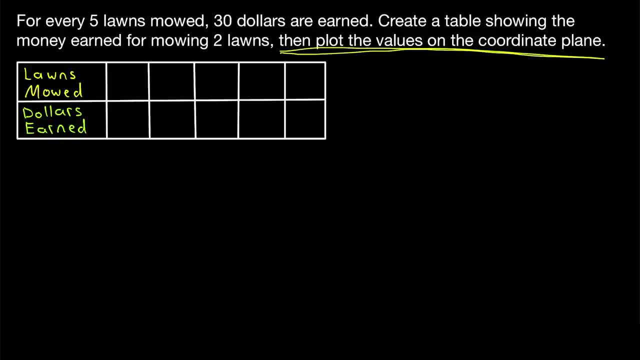 a student giving this question, I would complain, because this question is really ambiguous. it just says: Then plot the values on the coordinate plane, But we don't know what values it wants us to plot. we're only asked to find one specific value, which is the money earned for mowing two lawns. so what values are we supposed to? 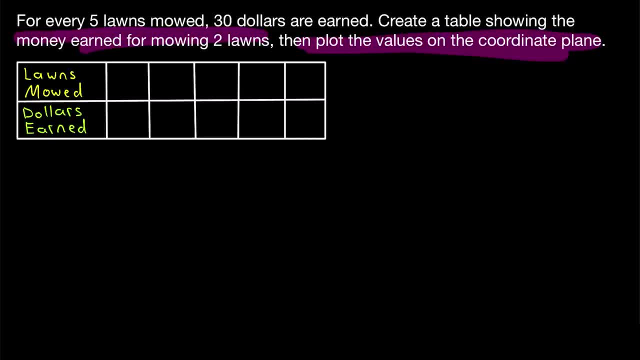 plot. well, thankfully, since I'm here narrating the video, I can decide that we're just going to plot whatever values we come up with while creating this table. all right, so the initial ratio we're given is that for five lawns mode, thirty dollars are earned. so that's a ratio. 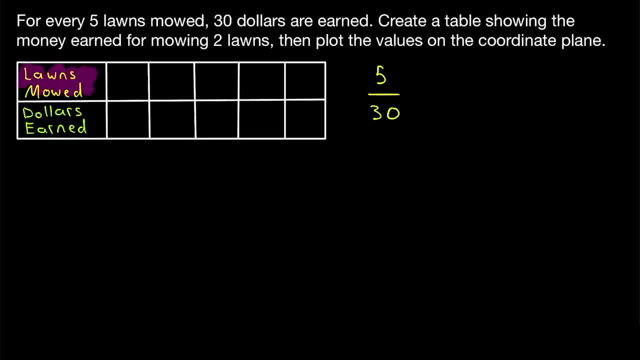 of five to thirty. We'll put the lawns mode Row first in our ratio table and then below that we have the dollars earned row. so we know if five lawns are mode will earn thirty dollars. I want to point out that in the previous 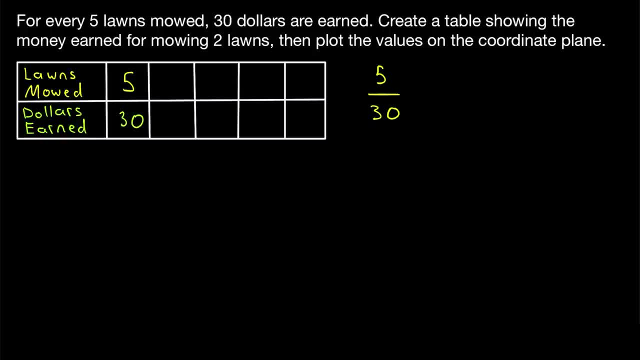 problem. we started off with what's called a unit ratio. that's a ratio that's given in terms of a single unit. in other words, one of the quantities should be one unit. ratios are very handy, but we don't have a unit ratio now, so let's try to scale this ratio down. 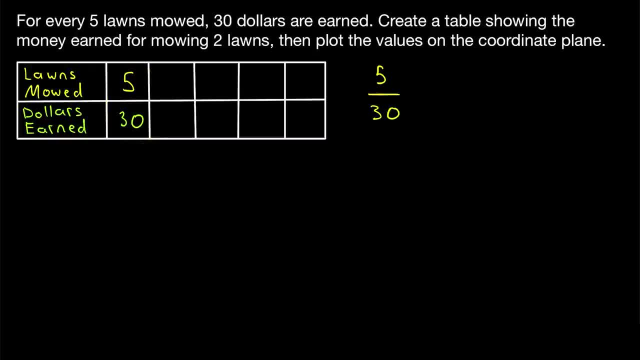 to A unit ratio. in order to change the numerator of our ratio to one, we would need to divide it by five. five divided by five is one. then to keep the ratios equivalent, we would need to divide the denominator by five as well. thirty divided by five is six, and then we 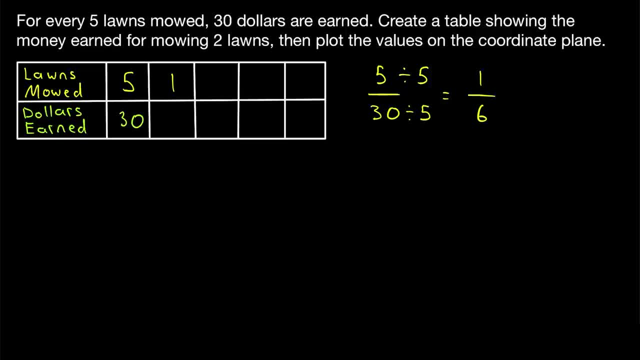 see, that is our unit ratio. so if we know one lawn will earn six dollars and we can put that in our table. now is a fine time to point out that we see, a ratio table does not have to be one or two lawns. the ratio table does not need to go up or down in any specific. 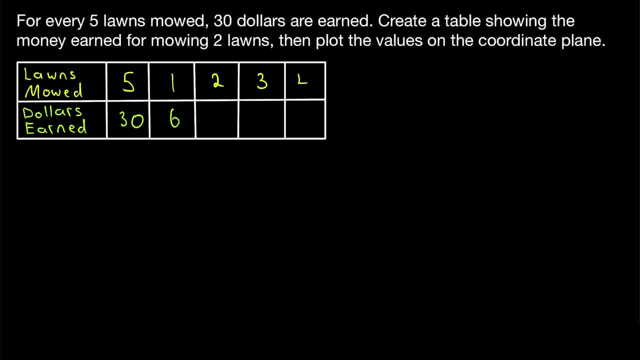 way. our values don't need to go one, two, three, four or anything like that. this is just a place to store information, so whatever information is useful for you to put in the table, you can put it in the table. the question is asking us to show the money earned for mowing two. 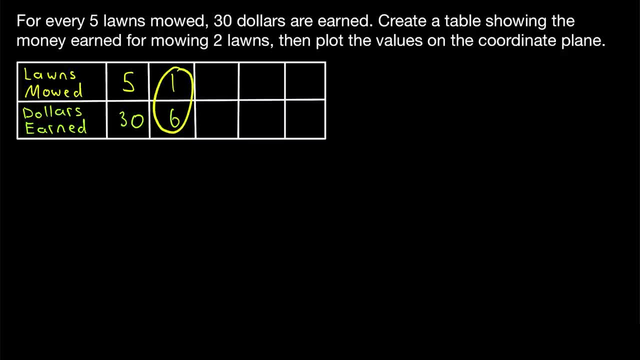 lawns. so now we'll want to scale our ratio up to two lawns, so we can multiply one lawn by two, and that's going to give us what we want: Two lawns, Two lawns. And then, to keep the ratio equivalent, we need to multiply six dollars by two as well, which. 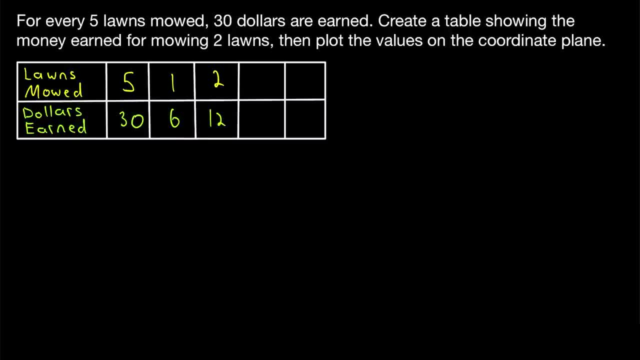 will give us twelve dollars now just for kicks. let's find one more additional ratio. what would we make if we mowed three lawns in order to find that number? we could scale our unit ratio up by a factor of three, or we could add these two ratios together, or we could 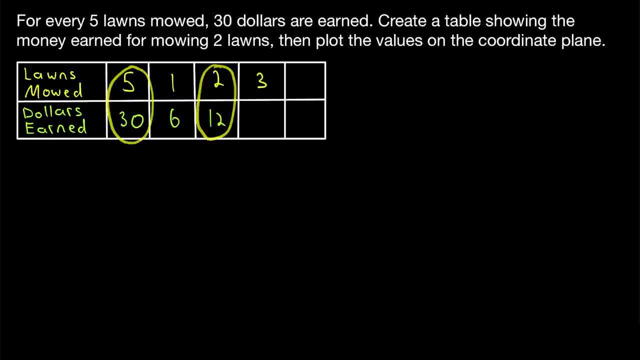 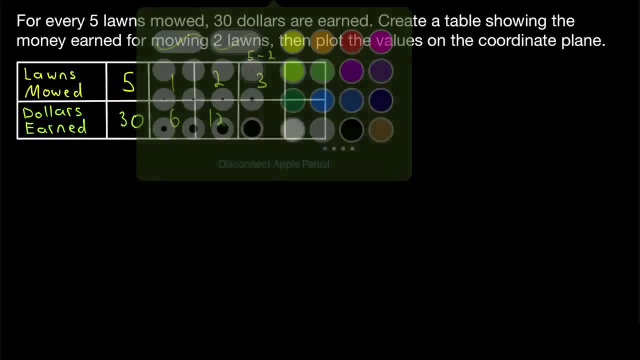 subtract this ratio from this ratio, Five lawns minus two lawns. Five lawns minus two lawns is three lawns. but if we mow two fewer lawns we know from our ratio that we're going to make twelve fewer dollars. so we would make thirty minus. 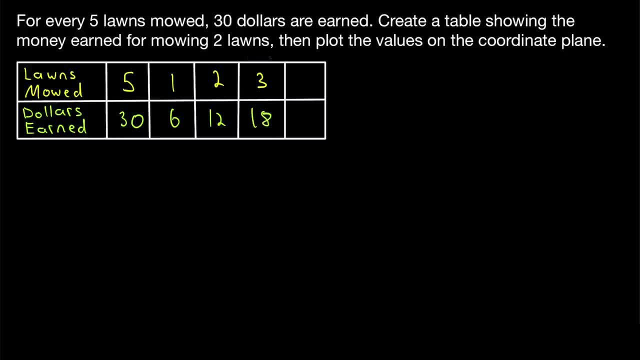 twelve or eighteen dollars. now I want to be very clear in this lesson. when we're talking about adding or subtracting ratios, we're not really adding or subtracting fractions. so we might express the five over thirty ratio as a fraction like this, and we might express 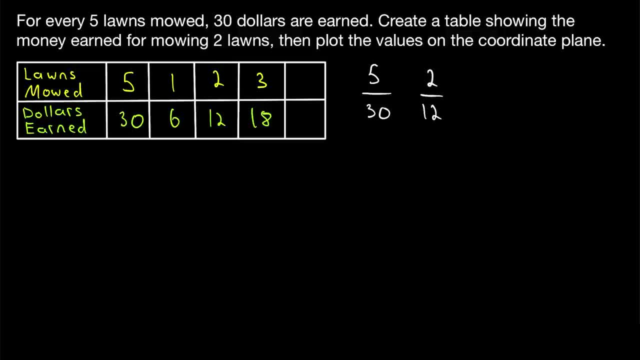 the two to twelve ratio as a fraction, like that. what we just did to get to a ratio of three to eighteen was not this, it was not the subtraction of fractions, because all of these ratios are equivalent. if we subtract, any two of them will actually always get zero. 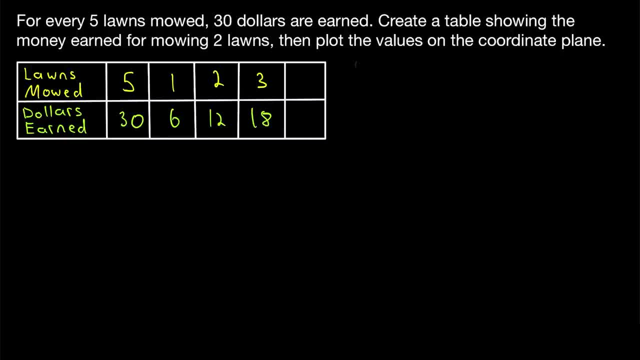 and same thing with the ratio addition we did above. if we quote on quote, add these two ratios to get to this ratio, We're not adding one sixth to two twelfths. instead, we're adding the individual quantities of lawns mowed and the individual quantities of dollars earned. and again, since all these, 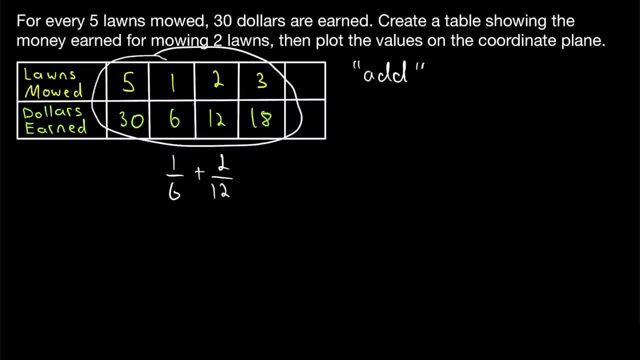 ratios are equivalent. in the same way that subtracting two of them would result in zero, adding two of them would just double them. so one sixth plus two twelfths, for example, is equal to two sixth, which is two times one sixth. It's also equal to four twelfths, which is two times two twelfths. I understand if this. 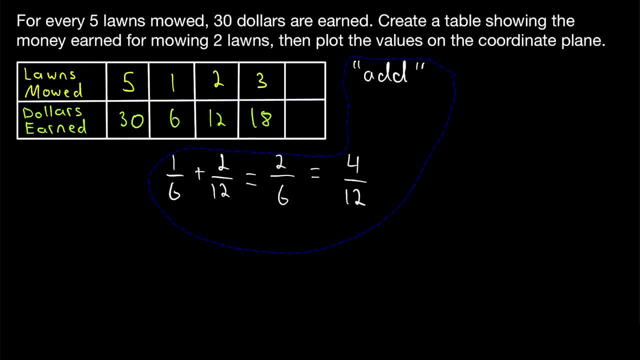 seems a little confusing and I encourage you to ask for any clarification you need down in the comments. now, to finish things up, let's just plot these values on the coordinate plane. our number of lawns mowed are one, two, three and five, so again going up by units of one. 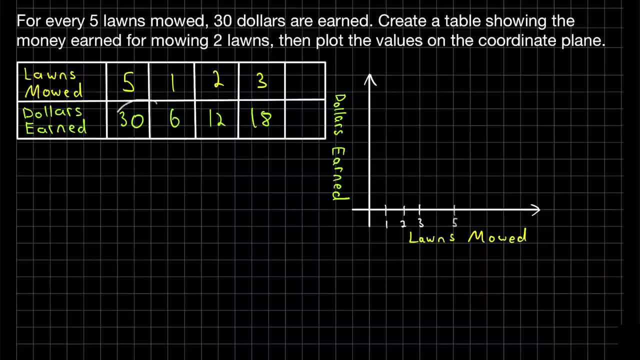 on the lawns mowed axis will work just fine. dollars earned, on the other hand, are going up by units of six. So we're going up by units of one. on the lawns mowed axis will work just fine. dollars earned, on the other hand, are going up by units of six. 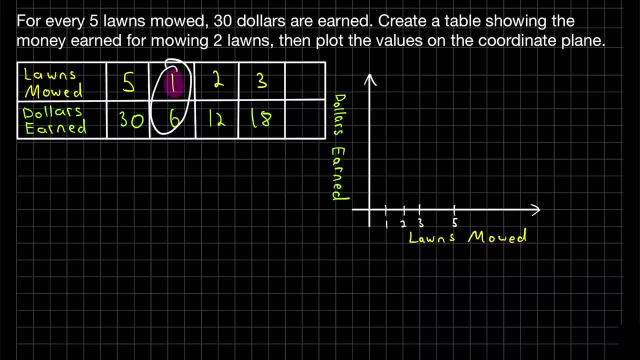 which we can tell from our unit ratio. for every one additional lawn mowed, we make an additional six dollars. so let's go up by units of six on the dollars earned axis and now we can plot the equivalent ratios. if we mow one lawn, we will make six dollars. so plot that point there. for two lawns, we'll make twelve dollars. for three lawns, we'll make eighteen dollars, and for five lawns we will make thirty dollars, and if it's bothering us, we'll make twenty dollars. 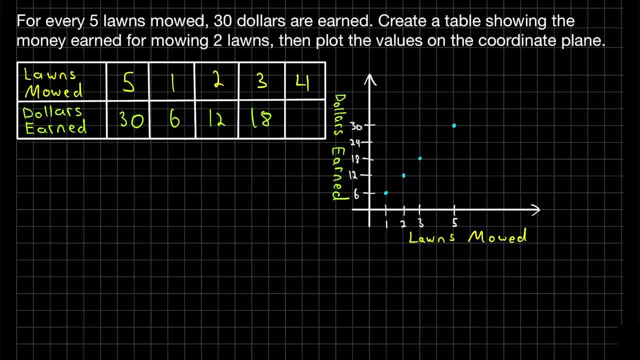 If it's bothering any of you, I suppose we can fill in the last column here. we can find out the number of dollars earned for mowing four lawns by simply doubling this ratio. so if we mow an additional two lawns to get to four lawns mowed, we would make an additional twelve dollars to get to twenty four dollars earned, and that would be this point right. here again we see that we can draw a straight line through these points, so we can be pretty confident they are indeed equivalent ratios. 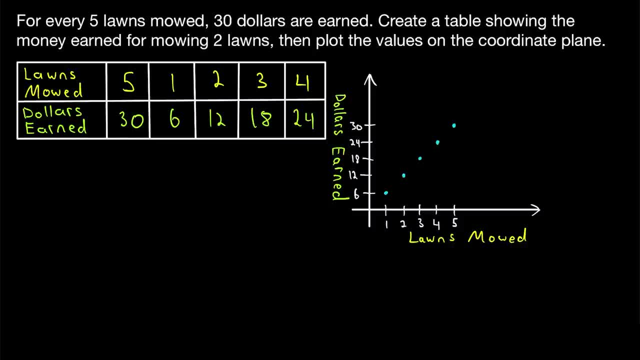 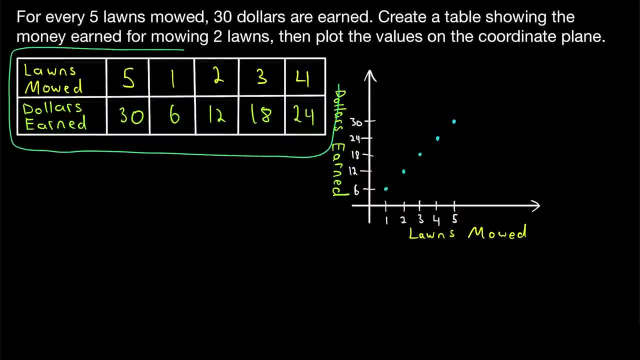 I know lots of you might be asked to do this stuff in a class. I just want to point out there's nothing special about ratio tables. we could easily get all of this information without a table and personally I would probably never use the table. It's just a way to organize your information. so if it's helpful for you and it helps you organize your thoughts and not make any mistakes, that's great and you should use it. but otherwise there's no particular reason to use it, unless you're being forced to for a grade. 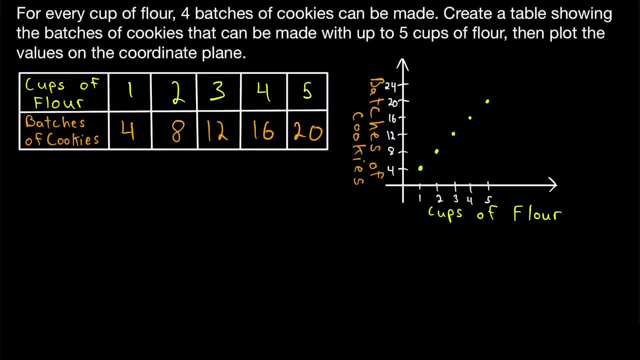 I hope this video was way longer than I expected. I hope it helped you understand how to create ratio tables and graph them in the coordinate plane. let me know in the comments if you have any questions, need anything clarified or have any other video requests. thank you very much for watching. I'll see you next time and be sure to subscribe for the swankiest math lessons on the internet.